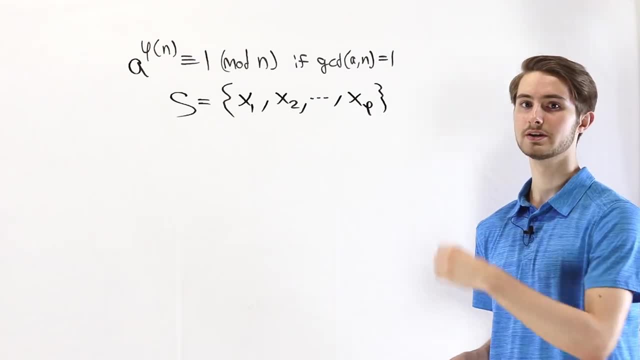 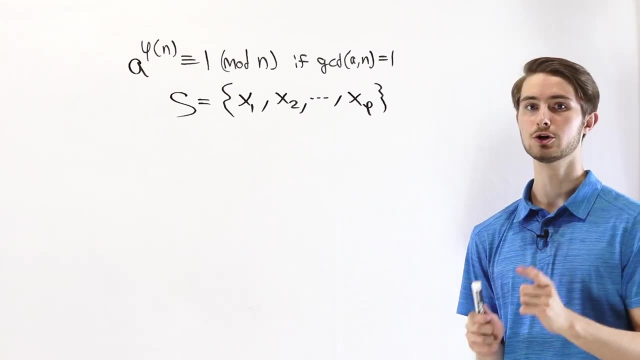 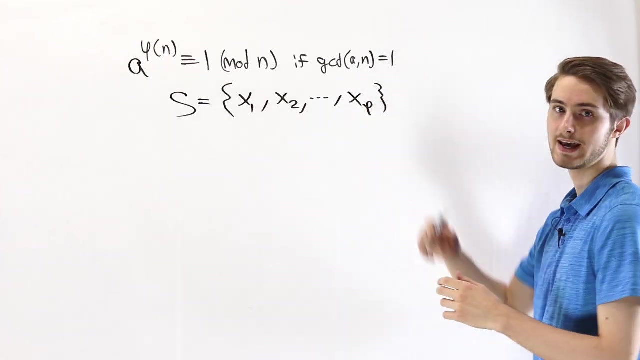 using the letter phi, because we know by definition that there are phi of n of these numbers. So these are all of the numbers from 1 to n that are co-prime to n. What we're going to do is take all of these numbers and multiply them by a. So let's see what happens if we do that. 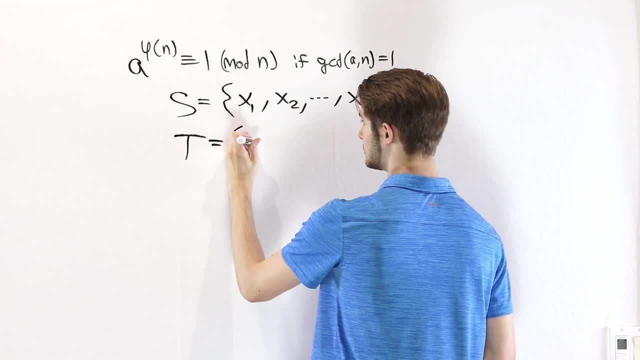 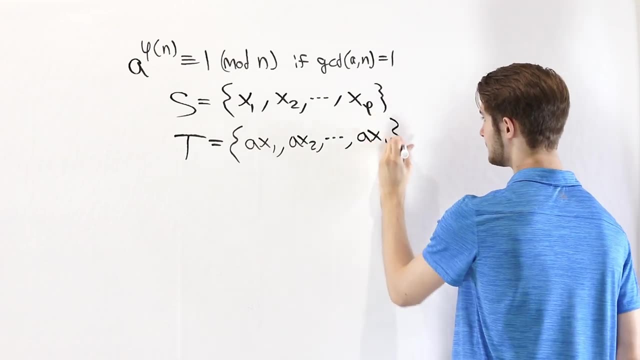 We're going to get a new set which we call t, and that's going to include ax1, ax2, and so on up to x phi. So these are the same numbers as we had before, but we're multiplying all of them. 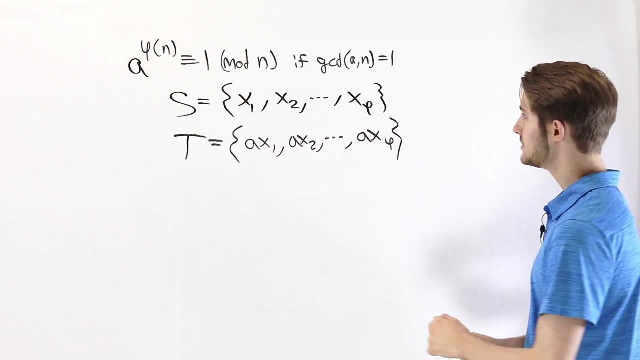 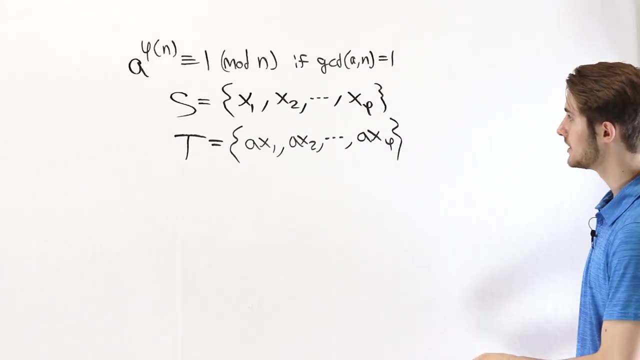 by the number a. We want to look at a few properties of how these two sets are related. First we're going to look at some properties of this set t. Remember that all of the x sub i's, all of the x's in this set here are co-prime to n by definition. 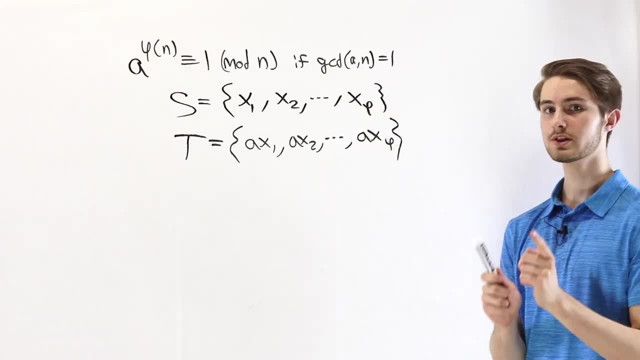 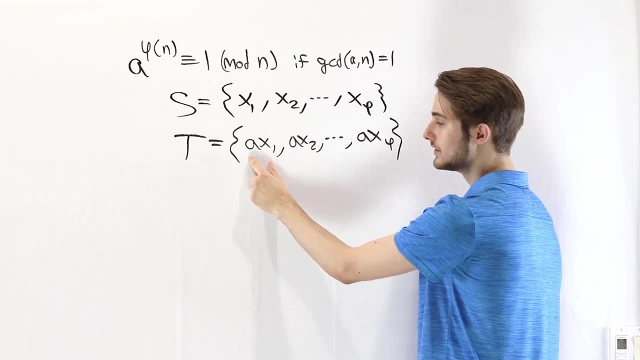 and we also know that a is co-prime to n. But one of the properties of co-prime numbers is that if a is co-prime to n and x1 is co-prime to n, then their product will also be co-prime to n. 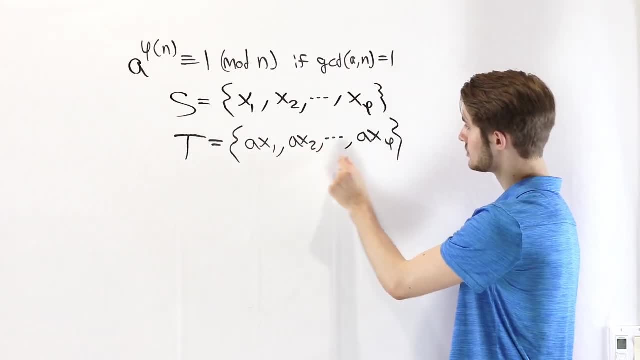 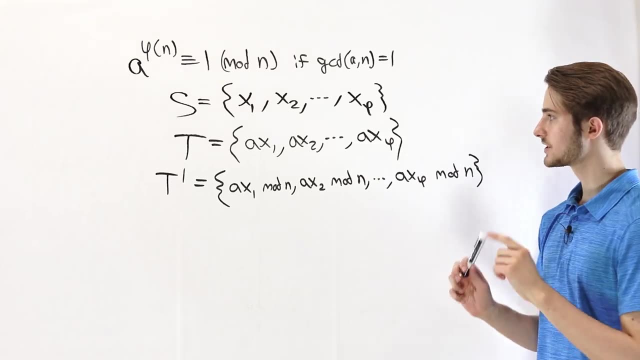 What that means is that ax1,, ax2, and so on, up to ax phi, all of these numbers are co-prime to n. Now we're going to construct another set, which we'll call t prime, and the way that we get t. 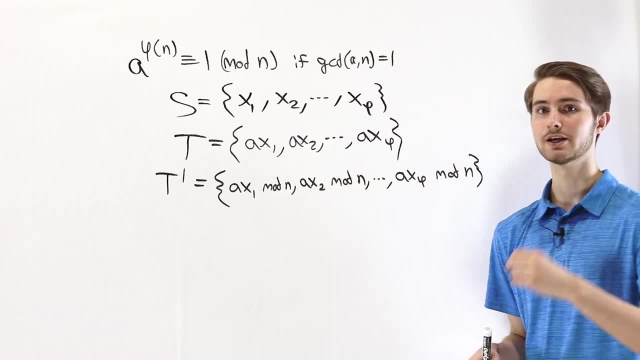 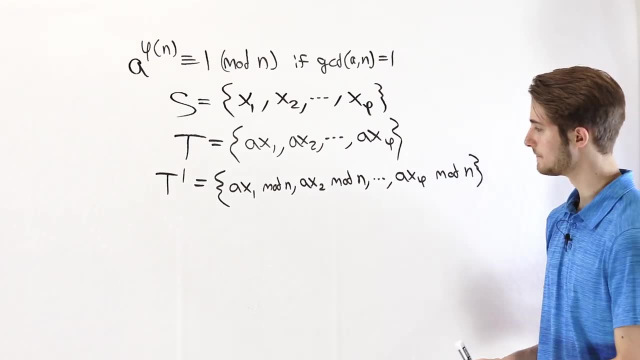 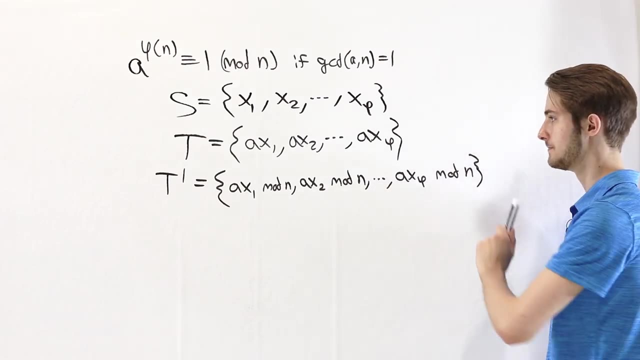 prime is by taking all of the elements of t and reducing them- mod n. Again, I talk about reducing numbers- mod n- in the video on co-prime numbers. So here we're looking at ax1, mod n, ax2, mod n and so on up to ax phi, mod n. Now there's another important property of co-prime numbers. 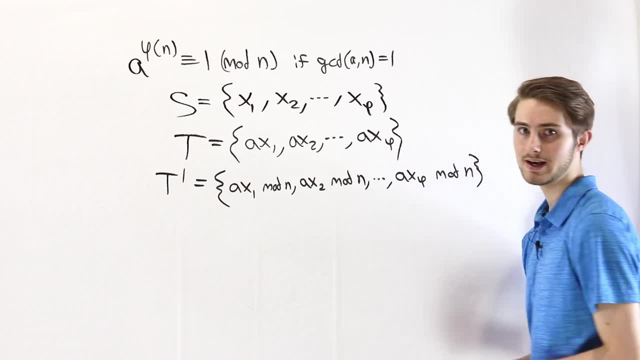 which says that if a number is co-prime to n, then when we reduce it mod n, this result will co-prime to n. So we're going to take all of the elements of t and reducing them mod n. Now there's another important property of co-prime numbers, which says that if a number is co-prime to n, 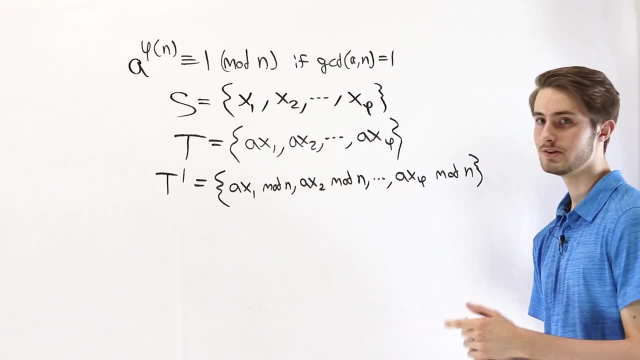 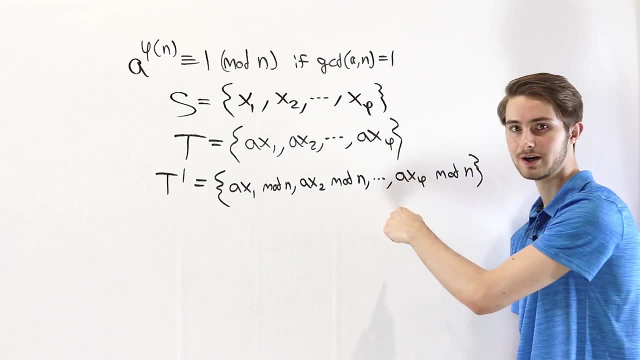 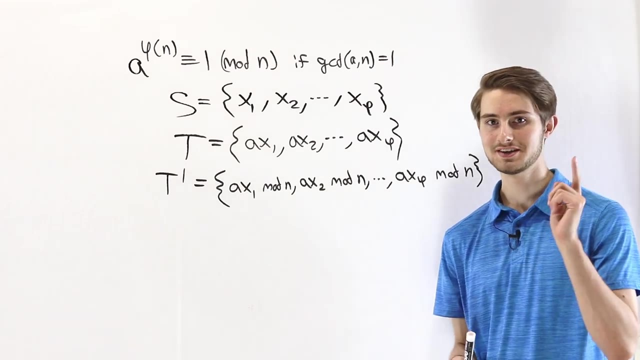 this result will still be co-prime to n. What that means is that because all of these numbers are co-prime to n, all of these numbers that we get by reducing mod n, these are all still co-prime to n. Now we're going to look at one more property that is key to the proof. Remember that there's a. 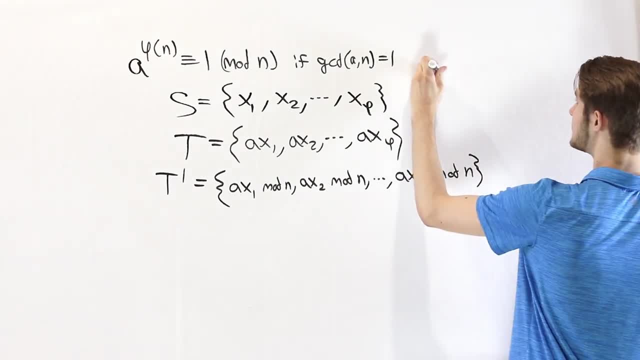 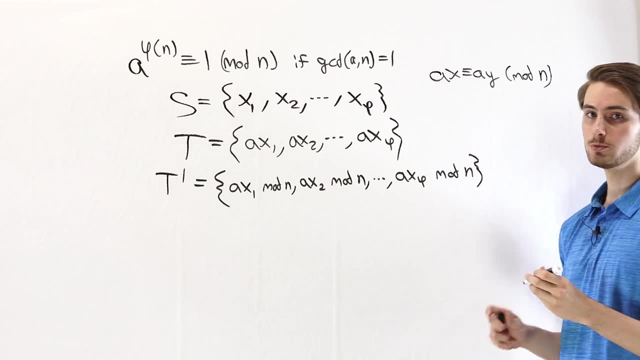 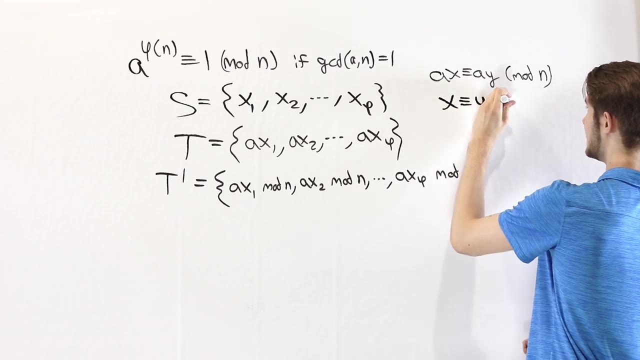 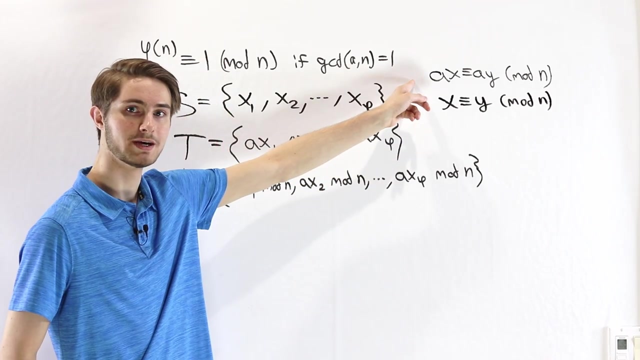 rule for cancelling numbers in modular arithmetic. If ax is congruent to ay mod n and we know that a is co-prime to n, then we can cancel a on both sides and get that x is congruent to y mod n. Now this has a very important consequence, which is that multiplying by 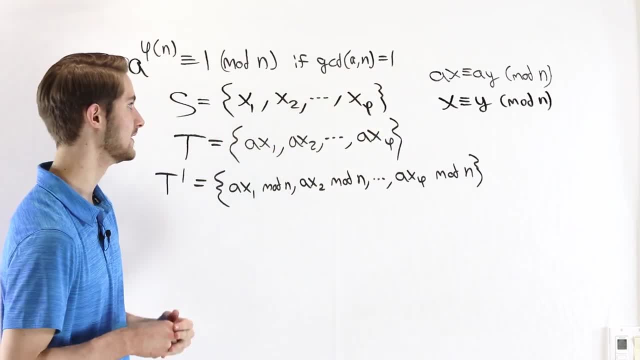 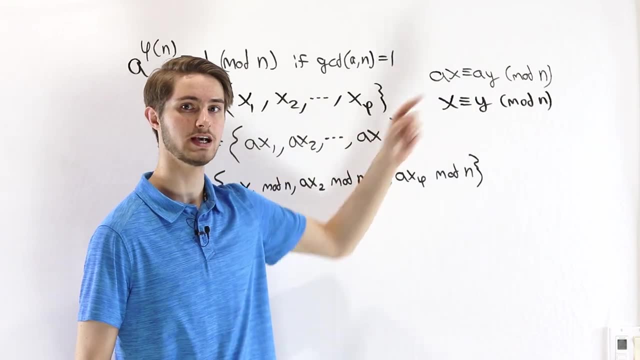 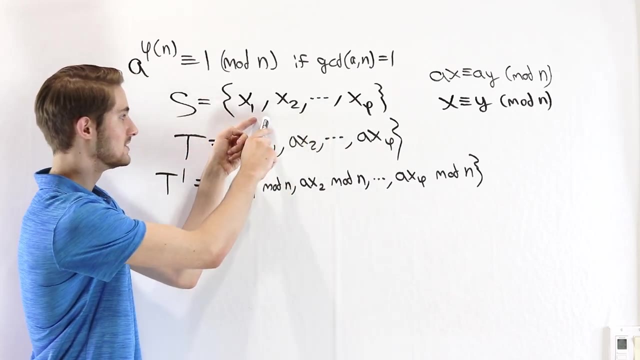 the number a is an injection, mod n. So if x is not congruent to y, then ax will not be congruent to ay, That's by the contrapositive. So what that means is that if x is congruent to y, then x is congruent to y. So what that means is we know all of these numbers in here. 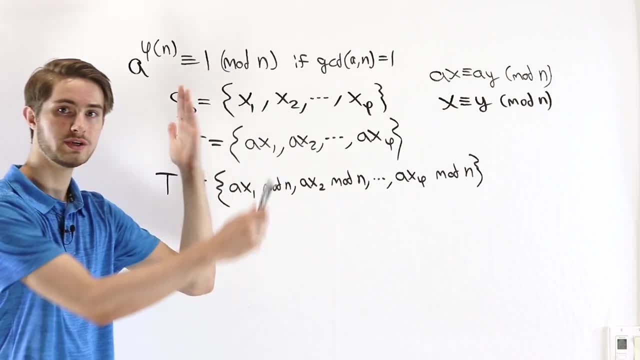 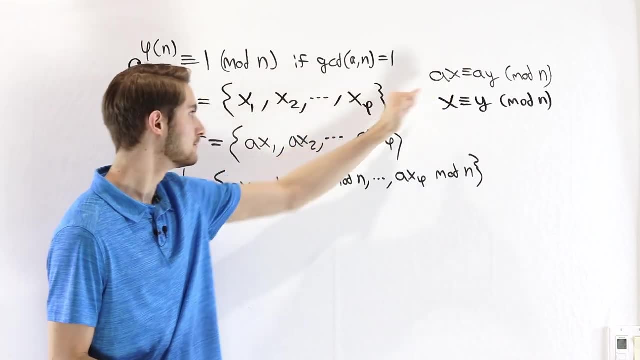 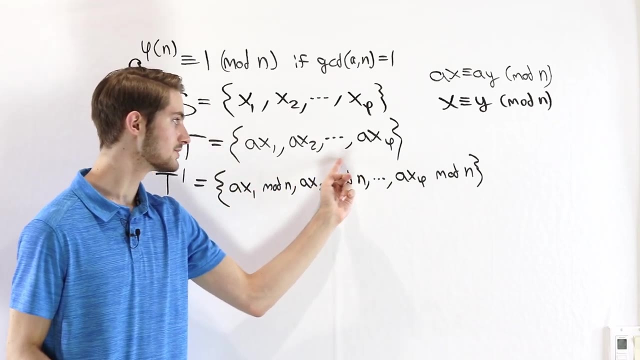 are not congruent. mod n because they're all between 1 and n. Now we get from s to t by multiplying the constant a. but if none of these numbers were congruent to mod n, then when we multiply by a, all of these numbers are still going to be incongruent. mod n because 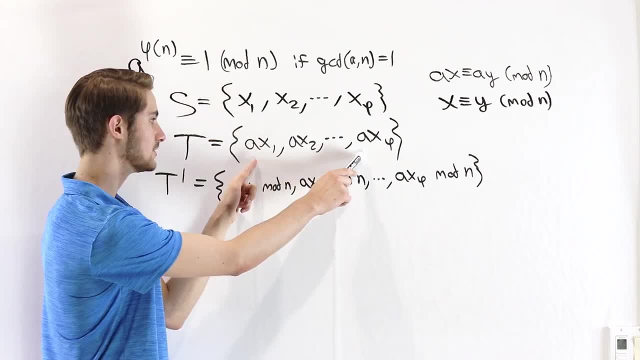 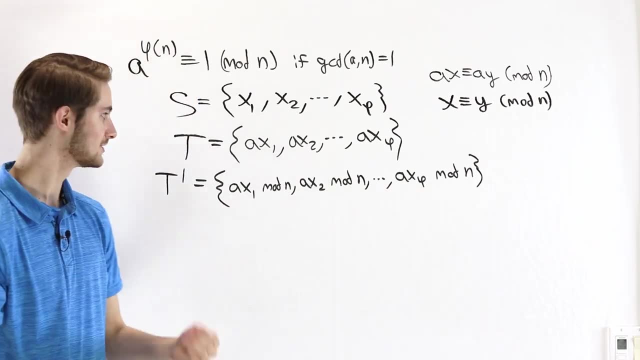 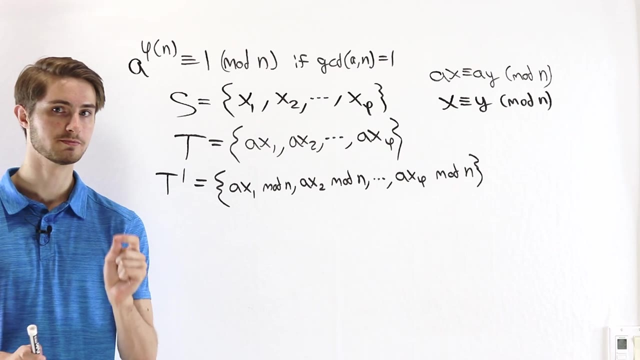 this is an injection, So these numbers are still all congruent to mod n, because they're all different mod n And when we reduce them, mod n- they're still going to be different. So these are all distinct numbers. Now we need to talk a little bit about reducing numbers. 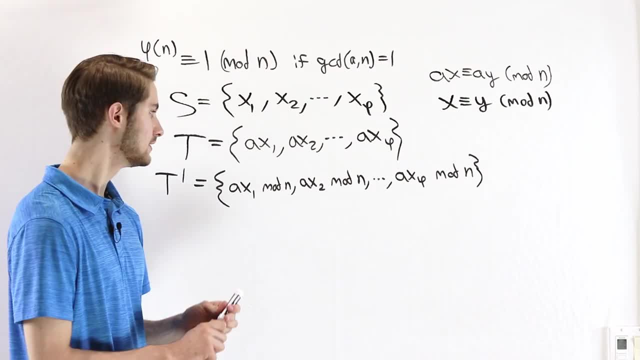 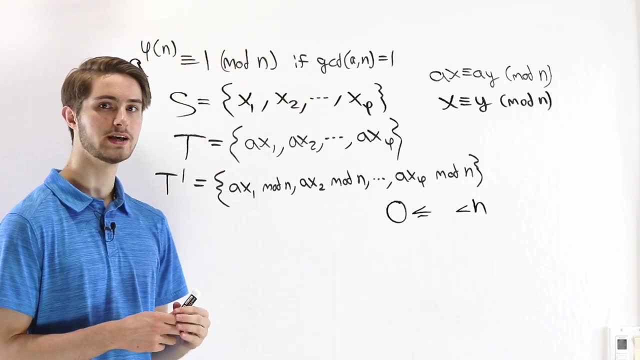 mod n. When we reduce a number mod n, the result that we get will always be between 0 and n, not including n. The reason for that is that if the result we get is bigger than n, for example, say, we're looking at n plus 2.. 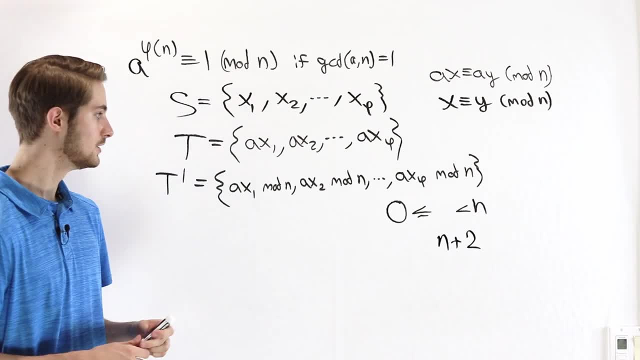 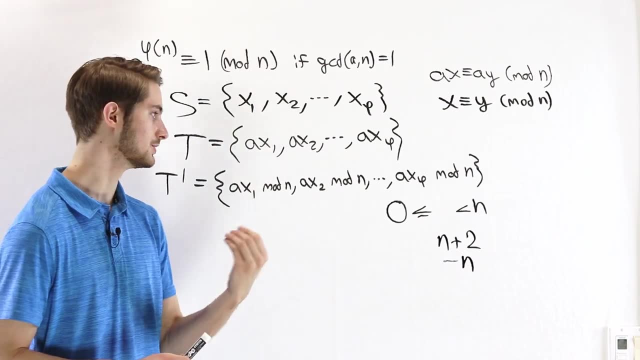 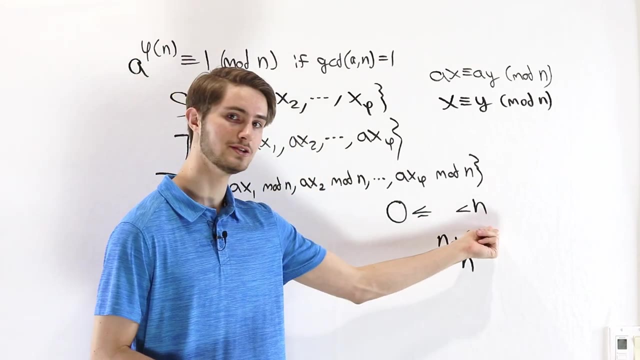 In that case, when we're reducing mod n, we could subtract another multiple of n and we would get a smaller integer that's still congruent mod n. So what that means is we can keep reducing the integer until it's in this range between 0 and n. So because all 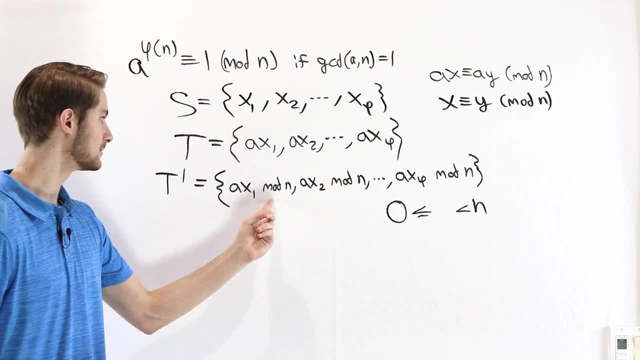 of these integers are the results from reducing a number, mod n. we know that all of these ax sub i must be between 0 and n. So if we were to get all of these integers out of the frame with the rest of the number, mod n, we would get a small number that's still congruent. 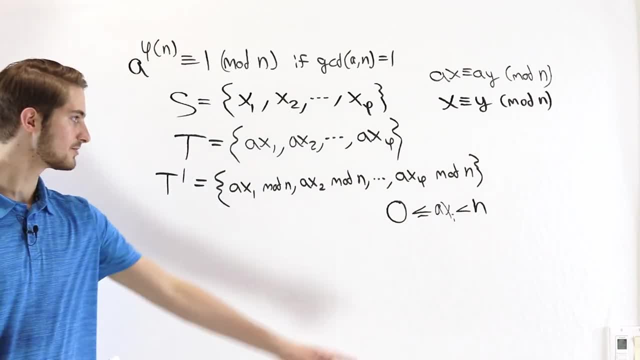 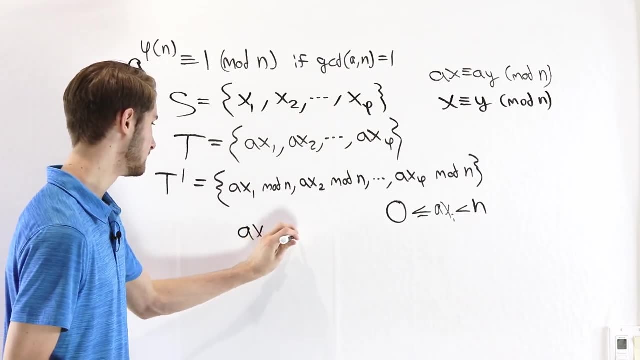 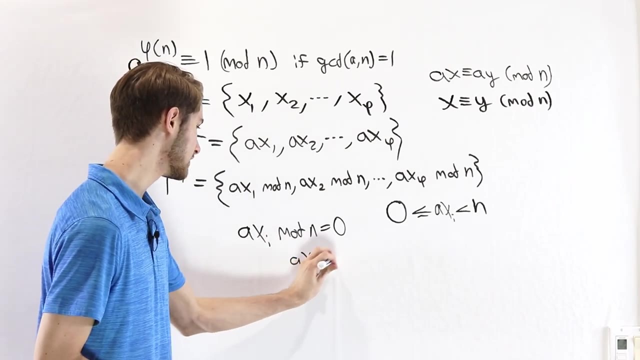 0 and n. In fact, we can go one step further than this. We can get more specific, because what would happen if a x i mod n were equal to 0?? Well, if that's true, then it means a x i is congruent to. 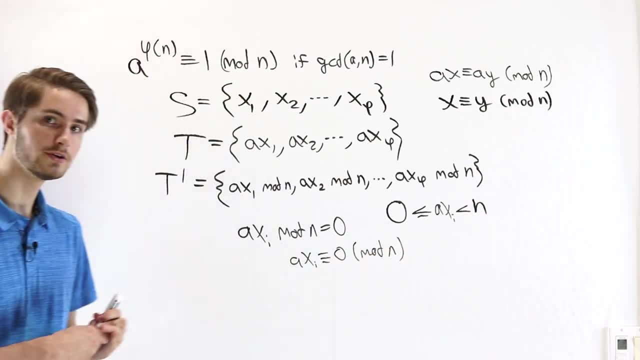 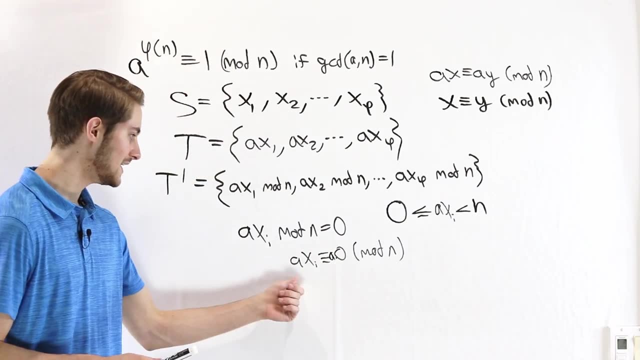 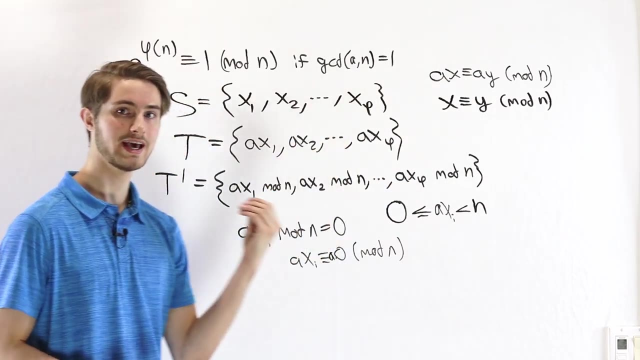 0 mod n. But notice that 0 is equal to a times 0. So we would have a times x sub i is congruent to a times 0. We can use the cancellation rule here. Of course, a is co-prime to n, so this would mean: 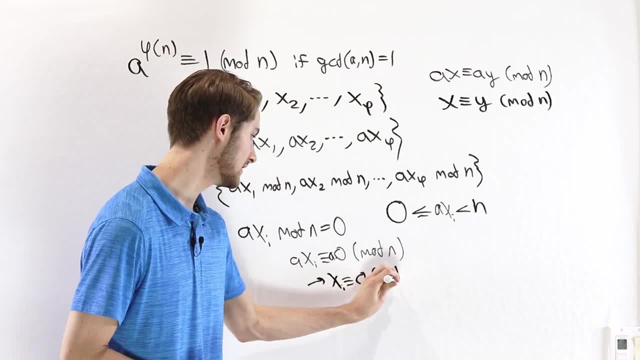 x i is congruent to 0 mod n. But we know that's not possible because all of these numbers are between 0 and n, So we can use the cancellation rule here. So if a x i is congruent to 0 mod n. 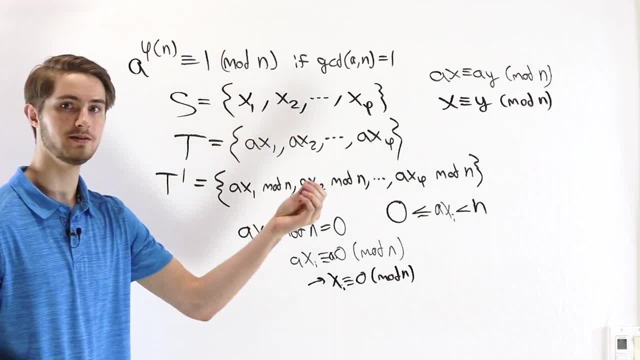 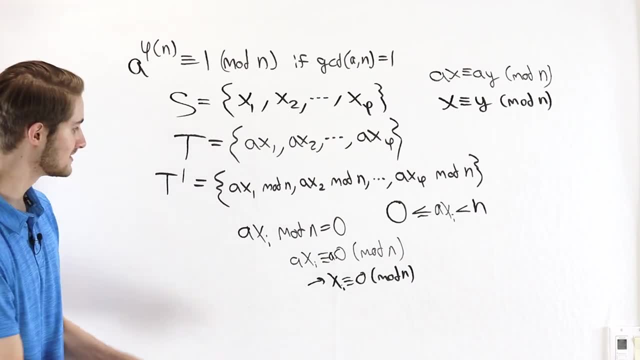 between 1 and n, and none of these x's are equal to n, because of course n is not co-prime to itself for any number greater than 1.. What that's telling us is: it's not possible to have a x i congruent. 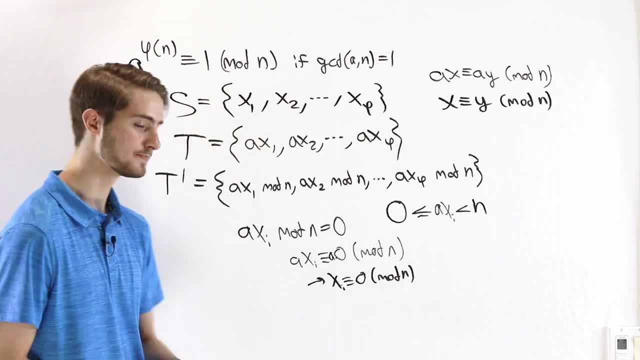 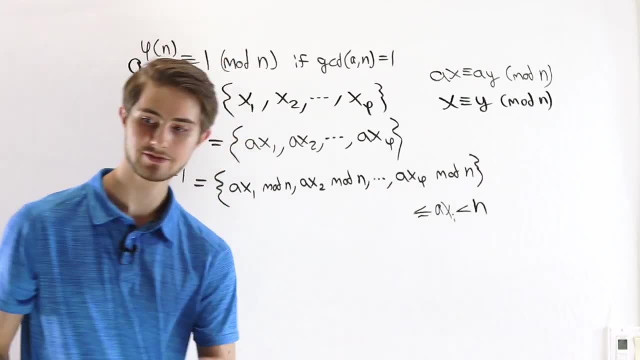 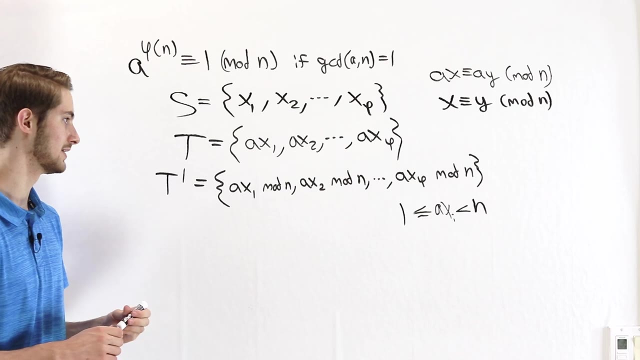 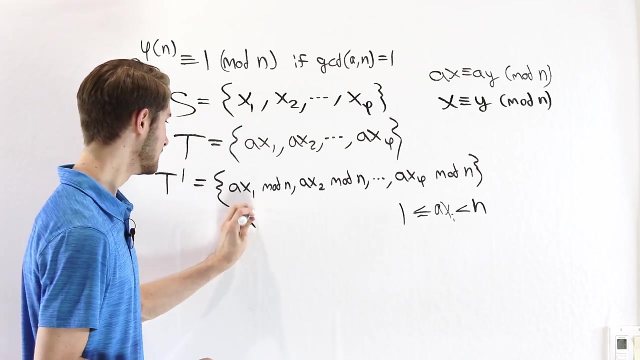 to 0, because that would contradict our original set. So 0 is not one of the possible values of t prime. They have to be between 1 and n. So let's think about the properties of t prime that we have right here We have a set of numbers between 1 and n. They are all. 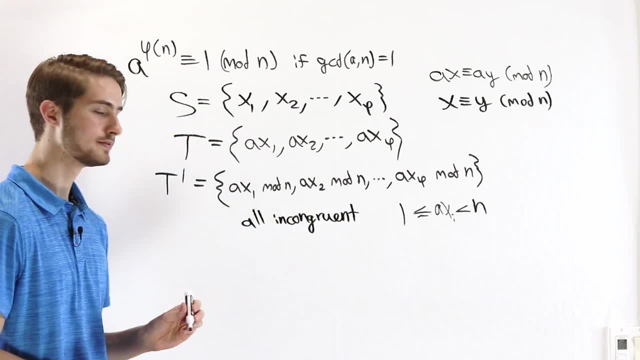 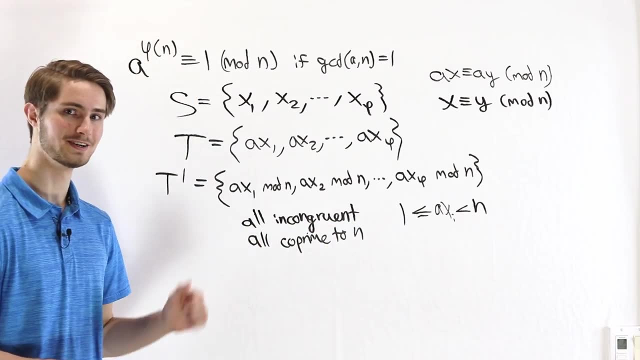 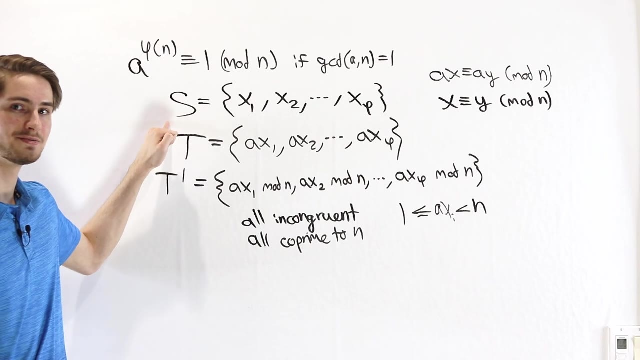 incongruent mod n, and they are also all co-prime to n. This is the fun part. These conditions should seem a little bit familiar, and that's because they're very similar to the conditions that we had on our original set S. All of these numbers. 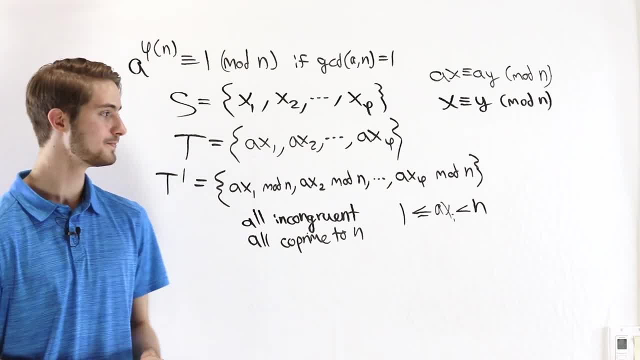 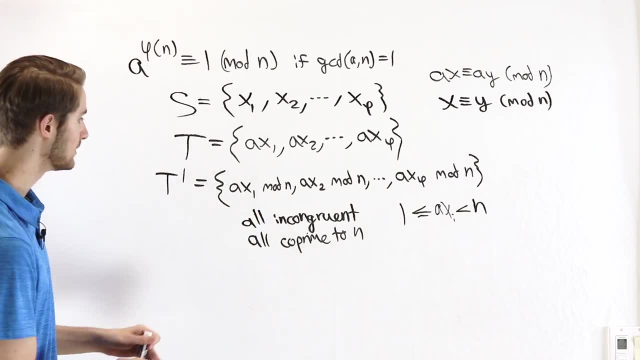 x1, x2, up to x, phi, those original numbers. those were numbers between 1 and n. They were all incongruent since they're different numbers and they were all co-prime to n. That's how we defined this set. These sets seem like they're pretty closely related, In fact. remember that. 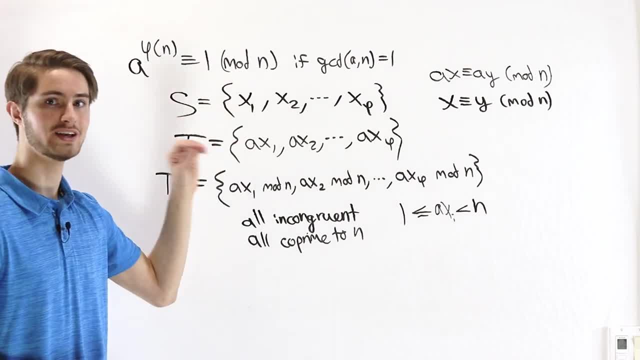 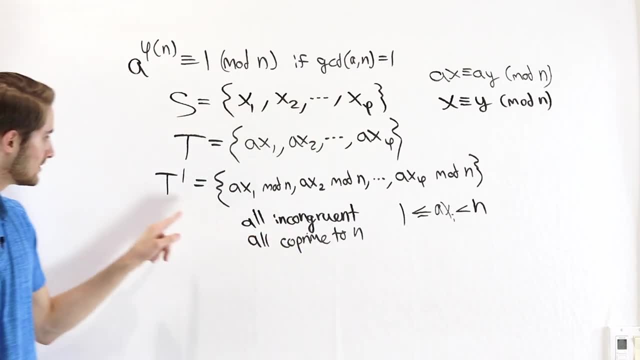 when we looked at S, we said these are all of the numbers, every single number between 1 and n. that's incongruent. and co-prime to n, And this last set here, t prime, has the same number of elements, since each element in 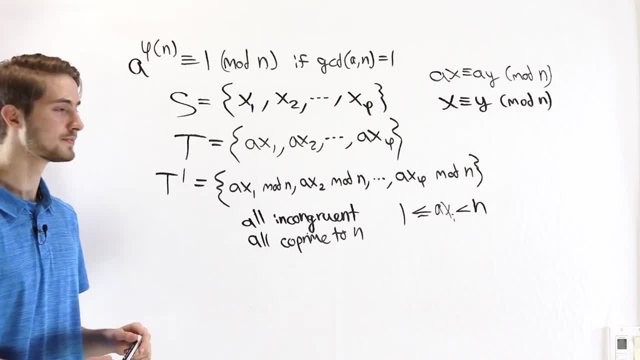 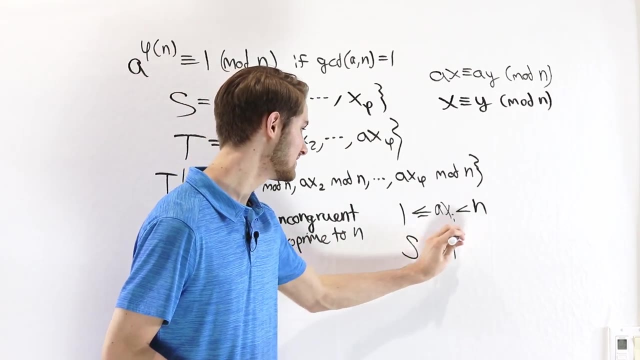 t prime comes from one of the elements in S. So if this original set contains all the numbers that satisfy these three conditions and t prime has the same number of elements that all satisfy those conditions, S has to have the same elements as t prime. They both. 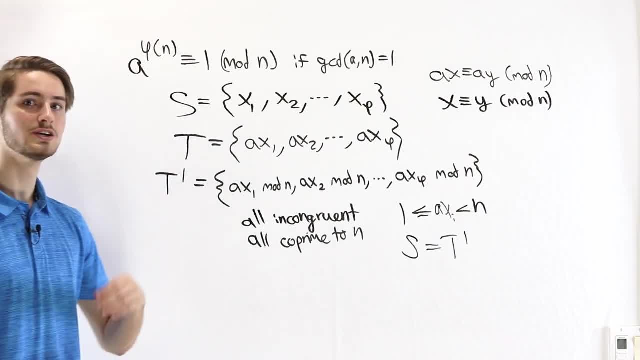 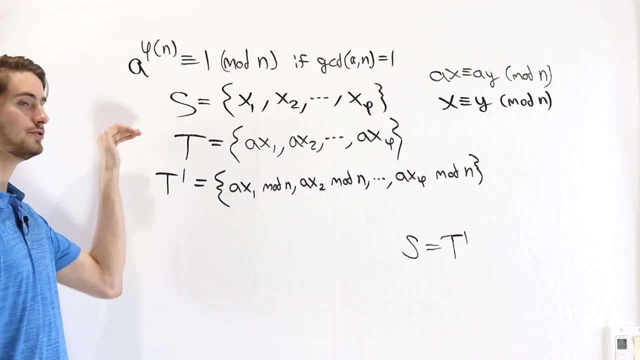 contain all of the elements that satisfy these conditions, So they have to have the same elements. Now remember that we got the elements of t prime by reducing the elements of t mod n. What does it mean to reduce a number mod n? Well, when we take 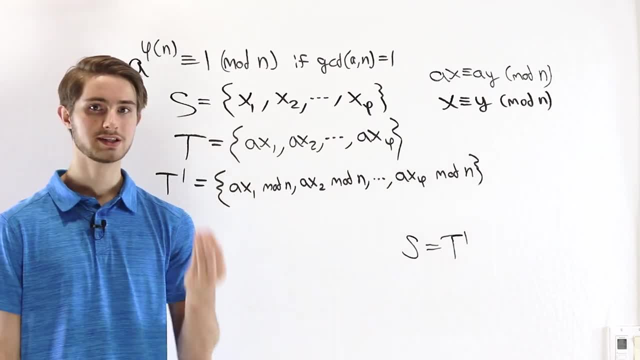 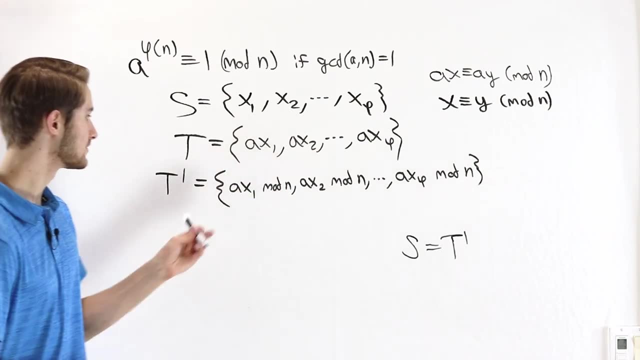 a number and reduce it mod n. the result we get is the least non-negative integer that's congruent to our original number, mod n. In other words, we can say that every number in t prime is congruent to one of the elements of t prime. So we have the same number of elements that satisfy these three. 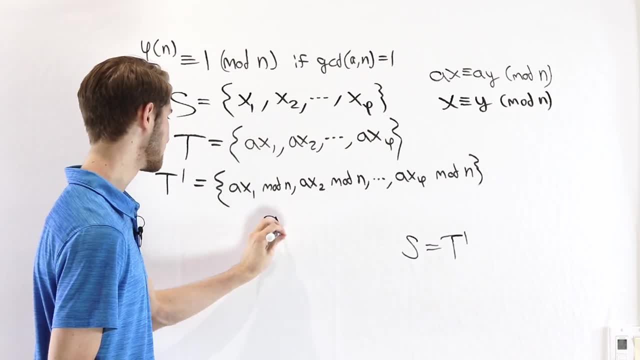 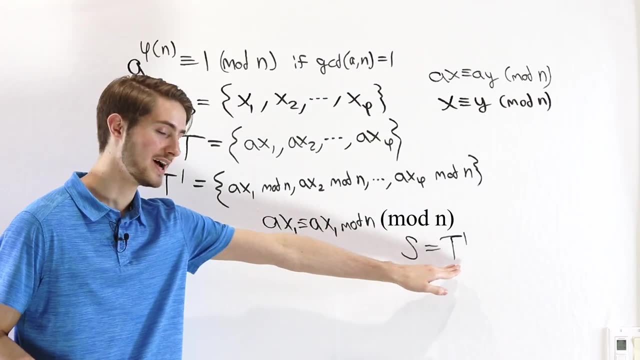 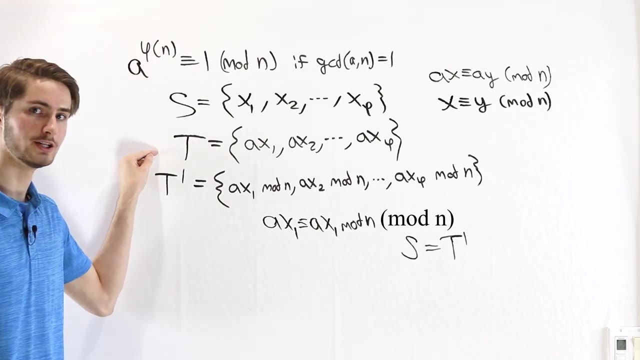 conditions. That's all I'm going to do now. but from here, remember that S has the same elements as t prime. So if every element in t prime is congruent to one element in t and S has the same elements as t prime, then every element in S is congruent to one element in t. Now, it might not necessarily. 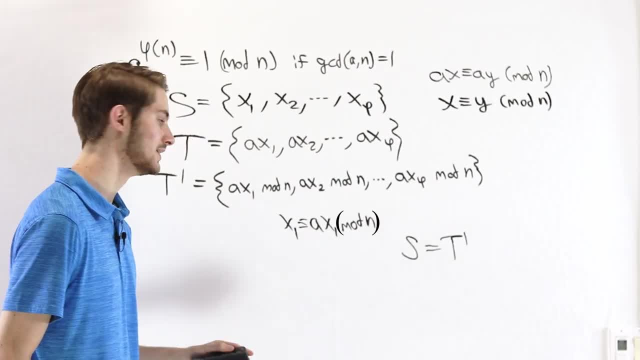 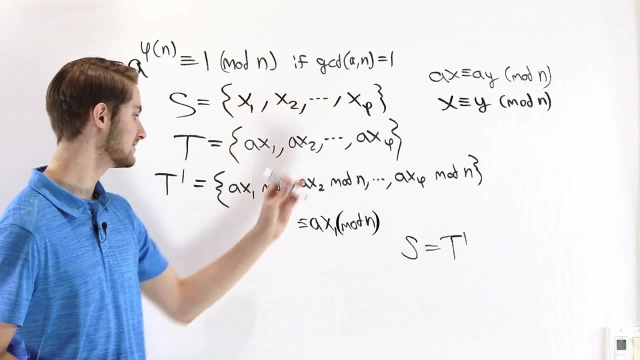 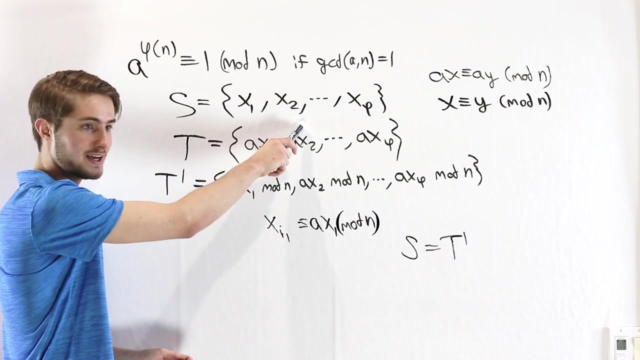 be the case that, for example, x1 is congruent to ax1 mod n. However, we know that there's going to be some number in this set. We'll call it x sub i1.. There's some number x in this original set that's congruent to ax1 mod n and this: 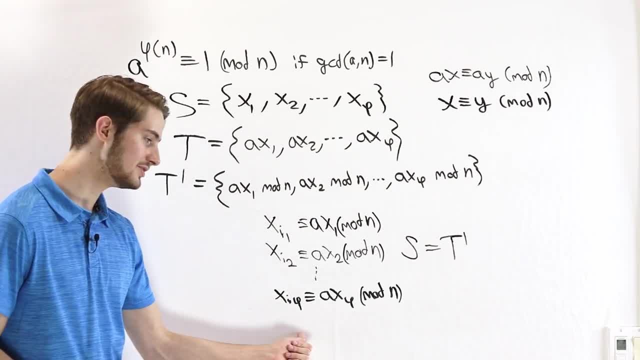 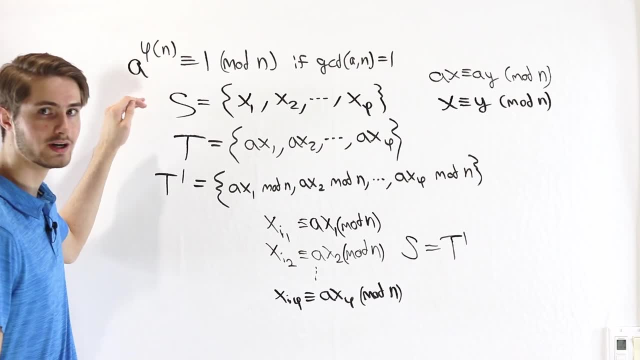 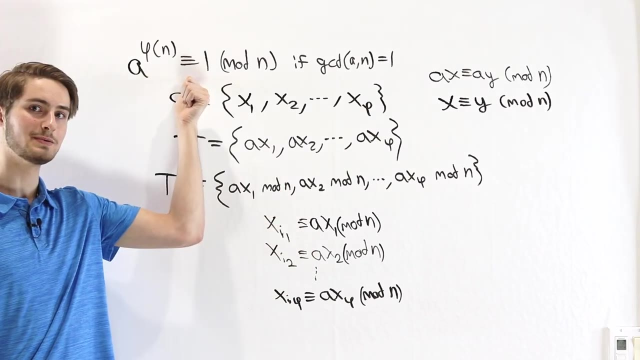 is true of every element all the way down to x, sub i phi being congruent to ax phi. Every single element in T is congruent to exactly one element in S. See if you can guess how we get from these congruences to the final statement. 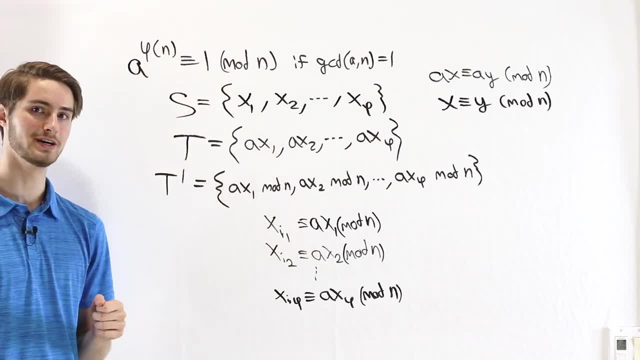 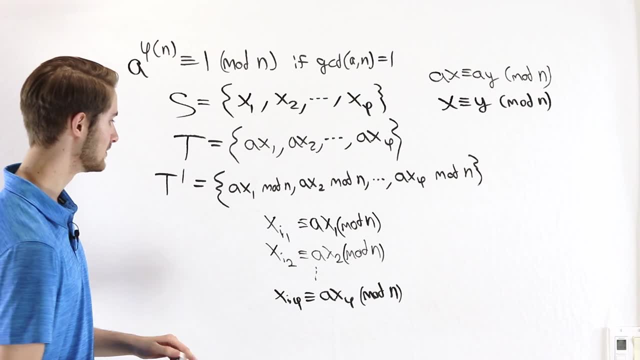 up here. a to the phi of n is congruent to 1 mod n. The way we're going to do that is using the multiplication rule for modular arithmetic. Remember that if we have two numbers that are congruent to each other- mod n- we can multiply the. 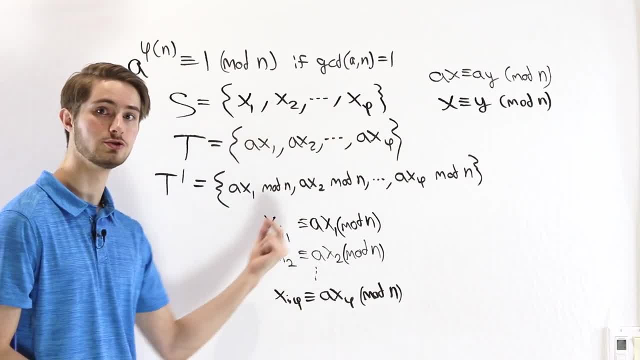 numbers from each of these two numbers, which is infinity into infinity. So let's numbers on the left and the numbers on the right, and those two products will be congruent. mod n. So what we're going to do is multiply all of the numbers on the. 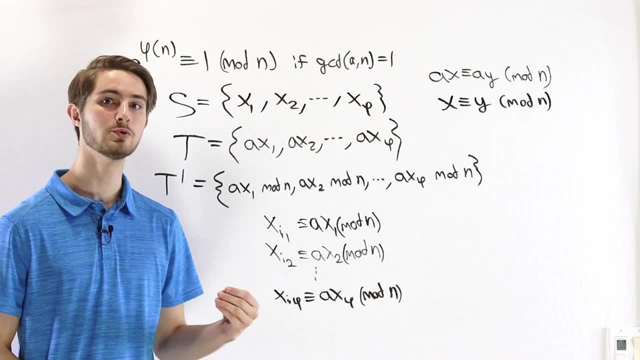 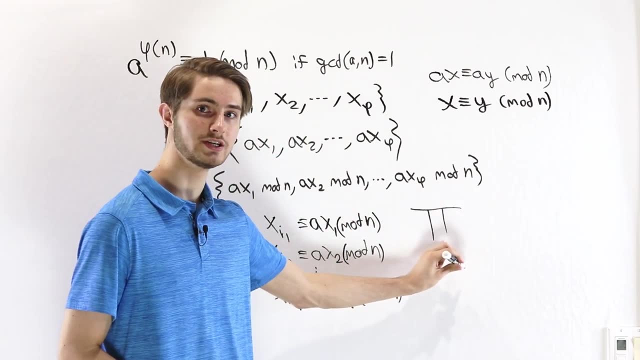 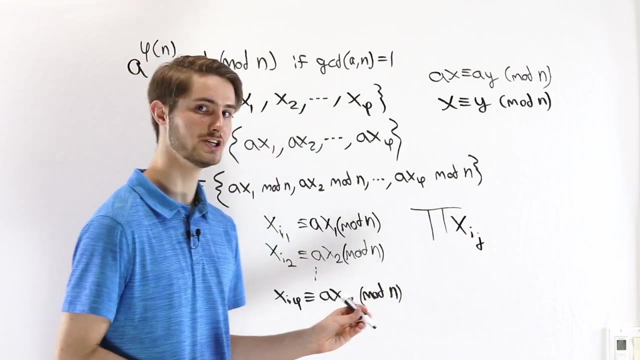 left with all the numbers on the right and see what products we get. On the left side we're going to get the product here. I'm using this notation here to talk about multiplying all the numbers: the product of x, sub i, sub j. That's going to. 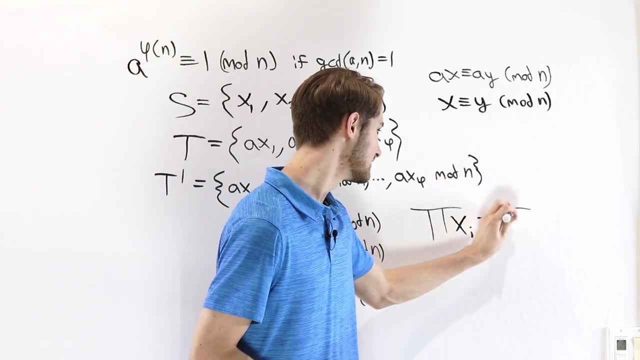 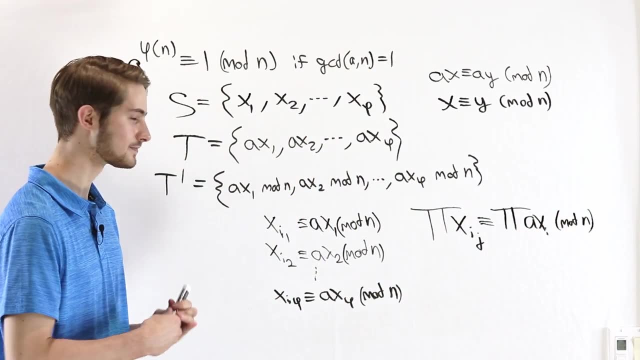 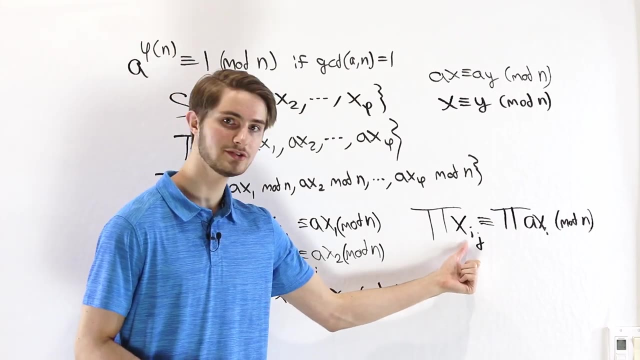 be congruent to over here, the product of all a x sub i. So these are all congruent mod n. Now remember that when we were looking at these x sub i1, x sub i2 and so on, all of these x's together, they were every single element in this. 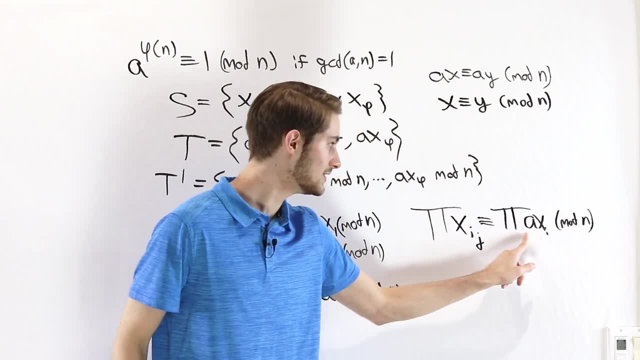 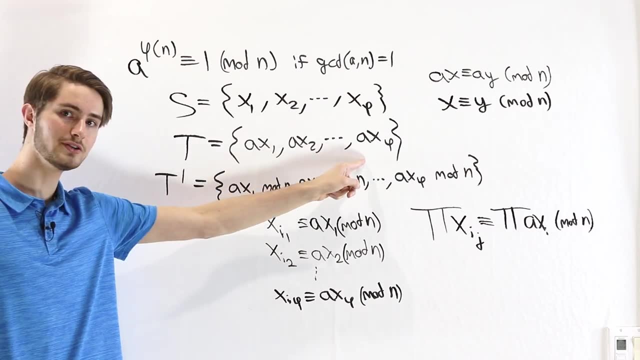 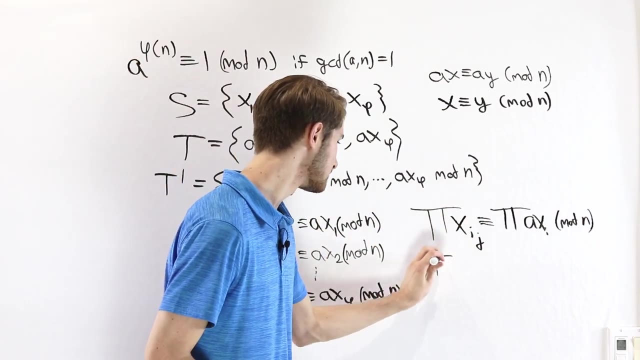 original set S. But all these numbers over here, a x sub i, these x sub i's we got from the set T And these are also all the x's in S. So these two products are the same products On both sides. we're looking at the product of x sub i, product of x sub i. 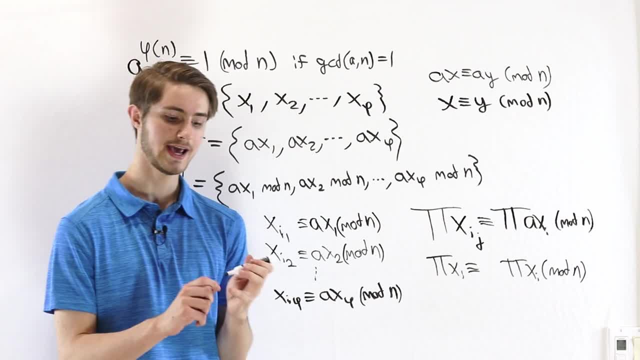 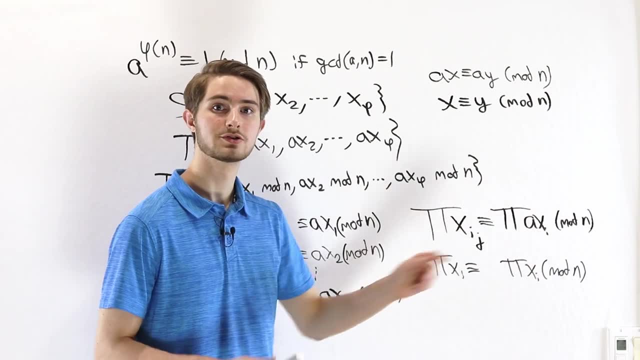 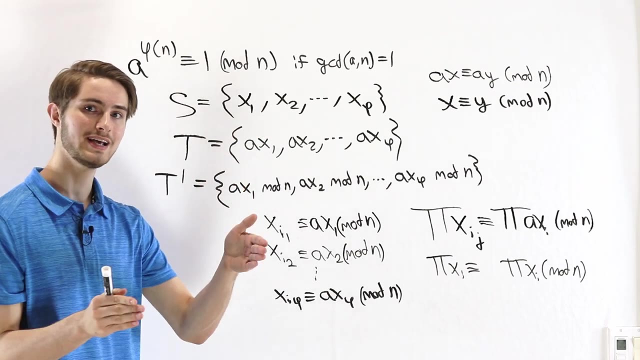 But then we have this extra factor of a and we're looking at the product. we're multiplying a over every single x sub i. So how many are there? Well, the number of x sub i is the number of integers between 1 and n that are co-prime to n, And by definition, that is. 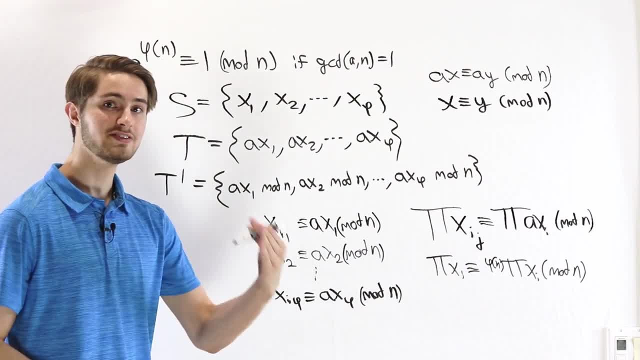 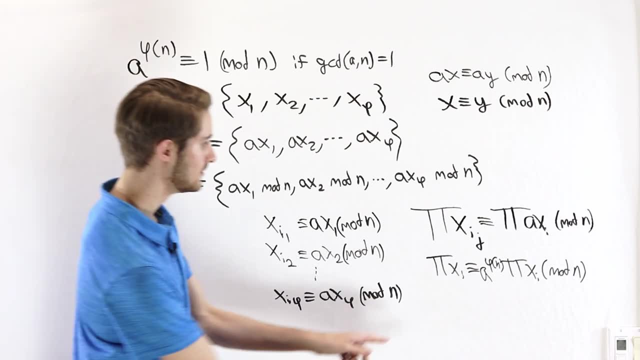 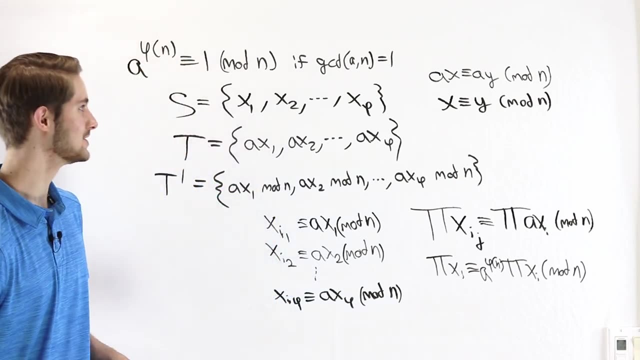 phi of n. So when we multiply phi of n copies of a, the result we're going to get is a to the power of phi of n. So these are congruent to mod n. But all of these x? i's are co-prime to n by definition, And we know there's a. 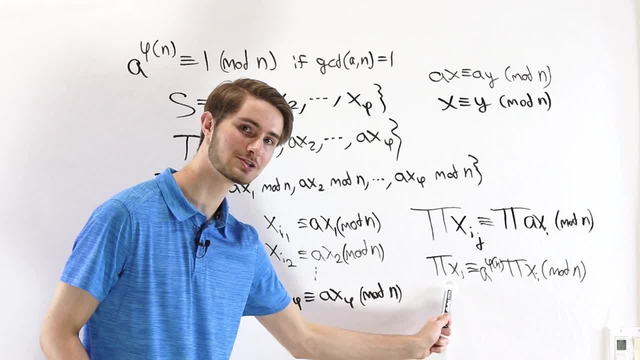 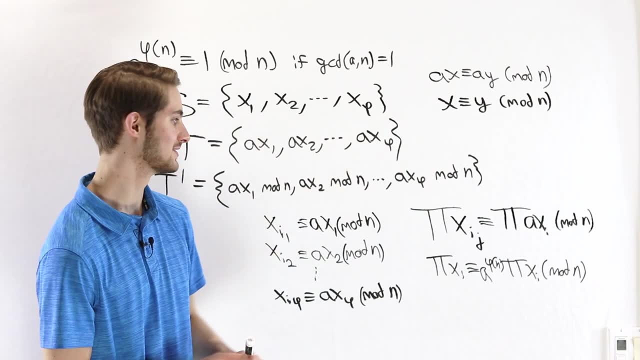 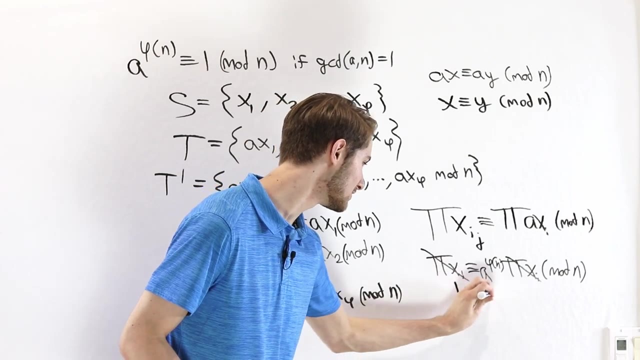 cancellation rule for modular arithmetic. If all these numbers are co-prime to n, their product is also co-prime to n, Which means we can cancel them on both sides. These two cancel out very nicely and we get the result. one is congruent to a to the phi. 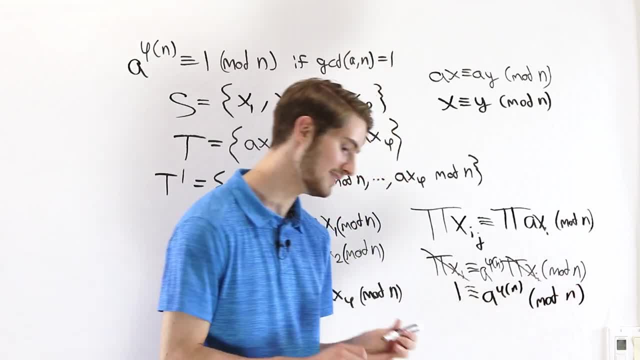 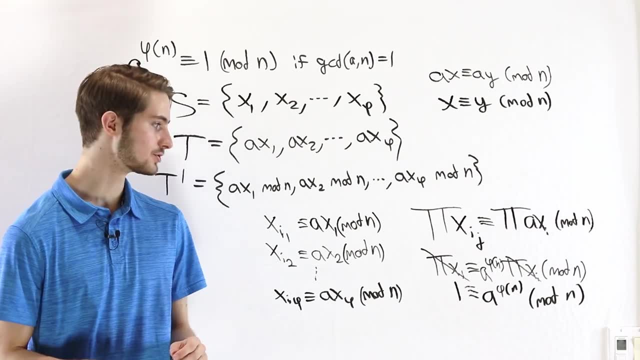 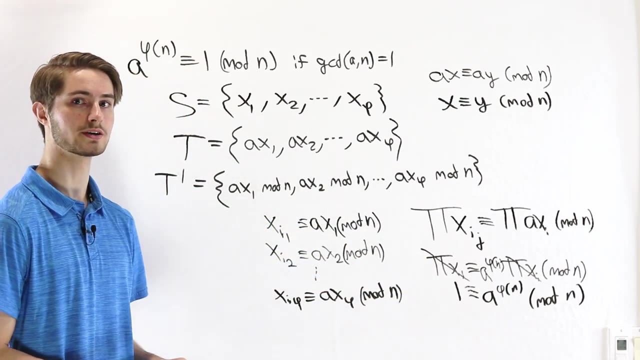 of n mod n, And that is Euler's Totion theorem. Now, when it comes to remembering why Euler's Totion theorem is true, I think it's easier, instead of looking at the final nice statement here, to look at the statement that includes the products, Because what Euler's 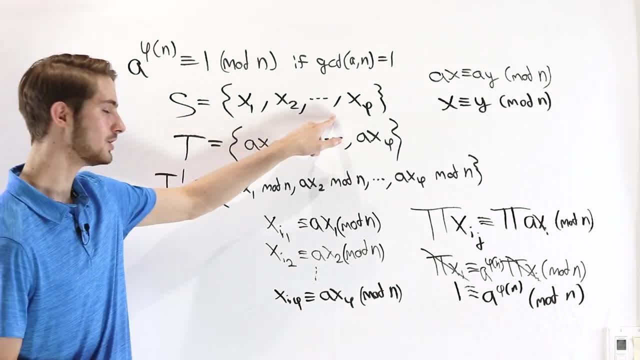 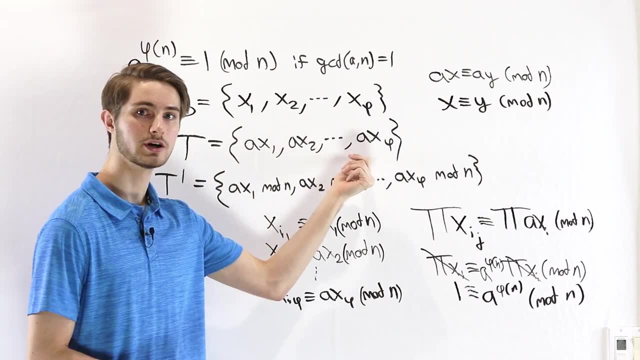 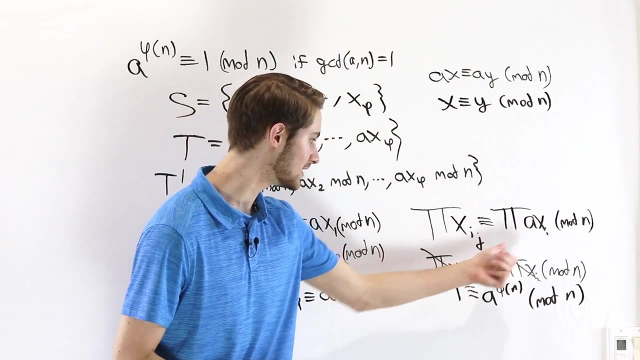 Toshin theorem is really saying is that if we take all the numbers co-prime to n and we multiply by a, the result that we get all of these numbers are going to be congruent to all the original numbers mod n in some order, Meaning that when we multiply them all together, those products are going to be. 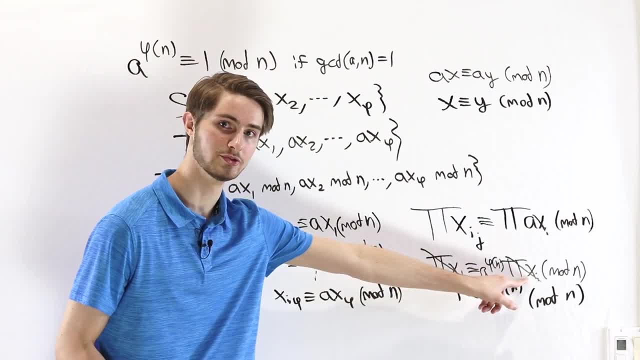 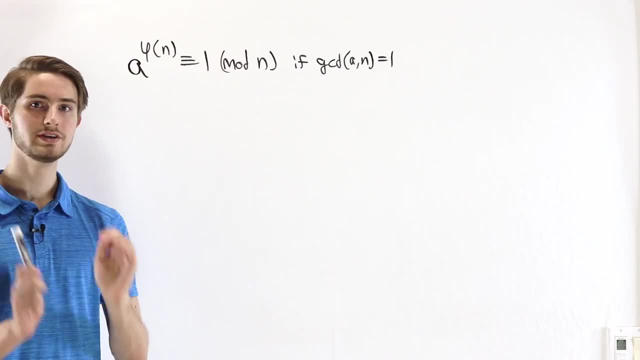 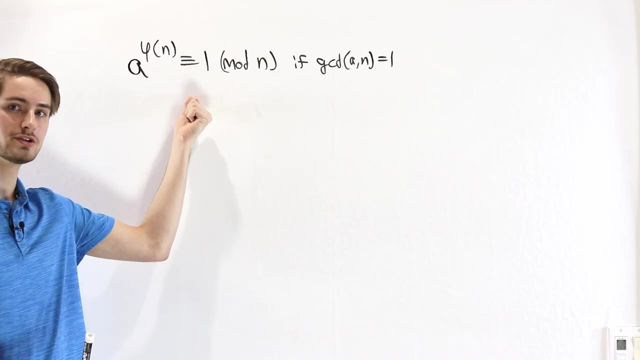 the same, And of course the products will cancel out on both sides and all we have left is phi of n copies of that number a that we multiplied. So now we're going to take a look at Fermat's Little Theorem. Now, Fermat's Little Theorem is actually a special case of this Toshin theorem. 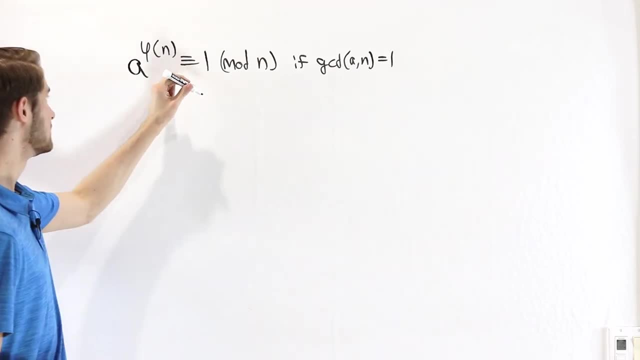 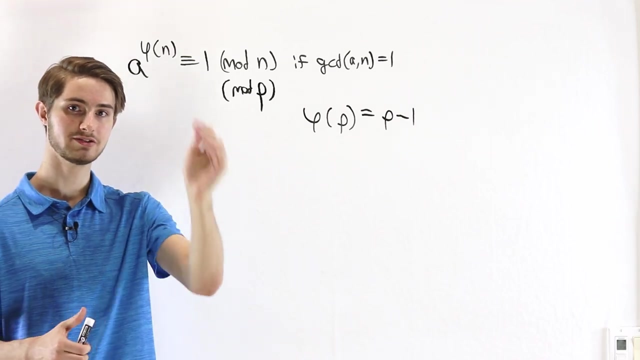 that we just derived, and it is the special case for when n is a prime number. So now we're working mod p. In that case, remember that the Toshin of a prime number, p, is equal to p minus one, because every number less than p is co-prime. 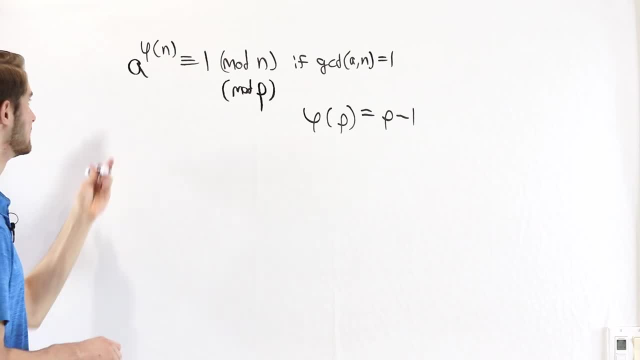 to p, And what that means is that up here in the exponent what we're going to get is p minus one. So a to the p minus one is congruent to one mod p. That's going to be true any time. a is co-prime. 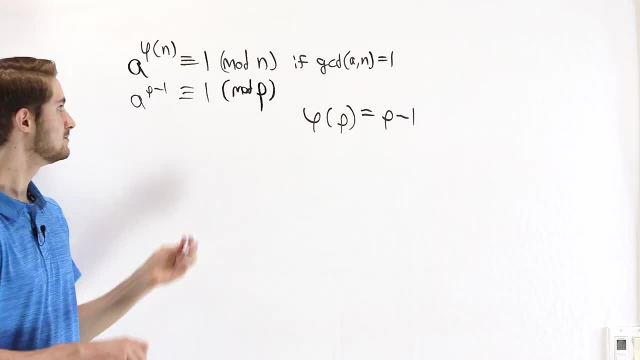 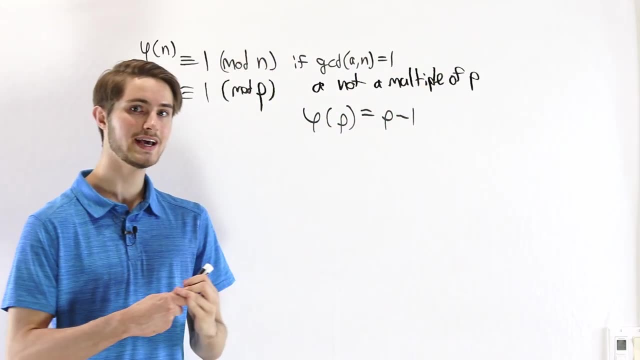 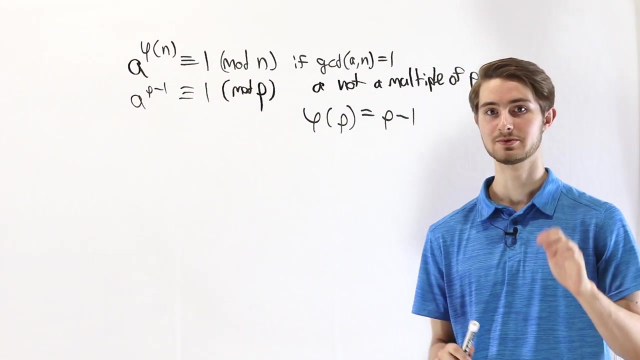 to p, And because p is prime, that just means we need a to not be a multiple of p. So as long as a isn't a multiple of p, this identity will be true. Now, the reason that we talk about Fermat's Little Theorem separately is that a lot of the time when we're doing modular, 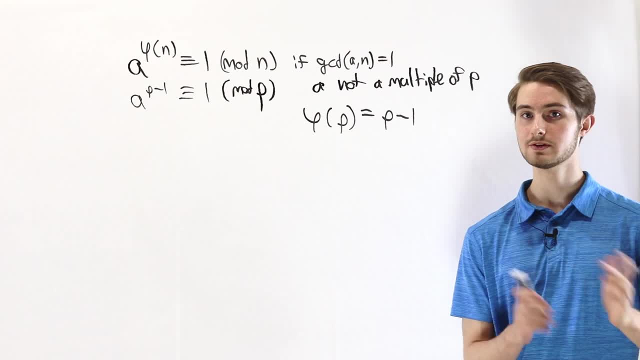 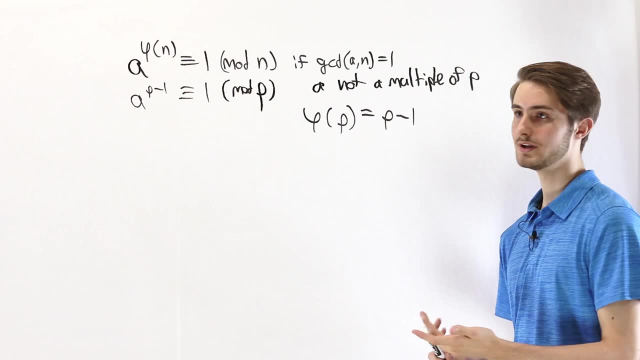 arithmetic, we're doing it mod a prime number. A lot of important ideas, such as primitive roots, come from the idea of doing arithmetic mod p. So it's important enough that it's easier to just remember that this specific identity a to the p minus one. 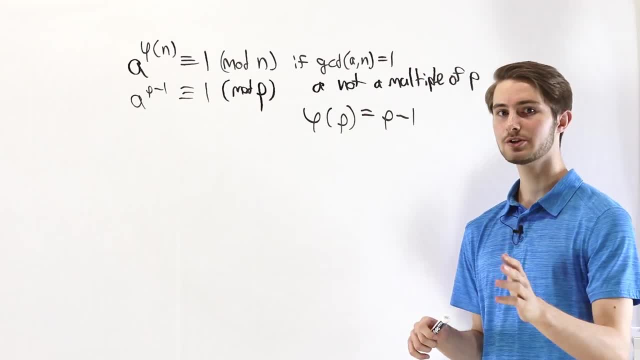 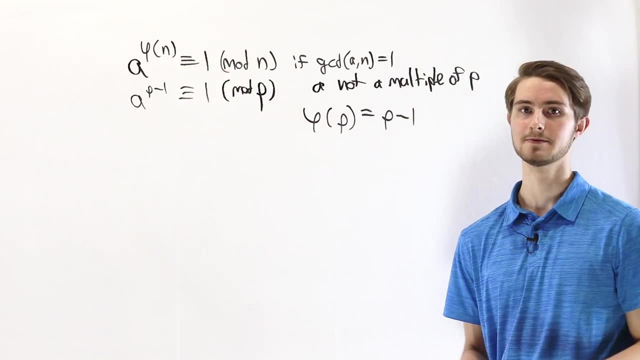 is congruent to one mod p. So that is Euler's Toshin Theorem and Fermat's Little Theorem. They both relate to taking exponents of numbers- mod n or mod p- And they have some very important applications further on in elementary number theory. 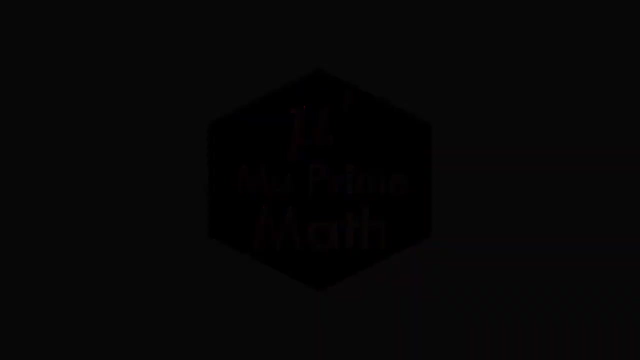 Euler's Toshin Theorem. 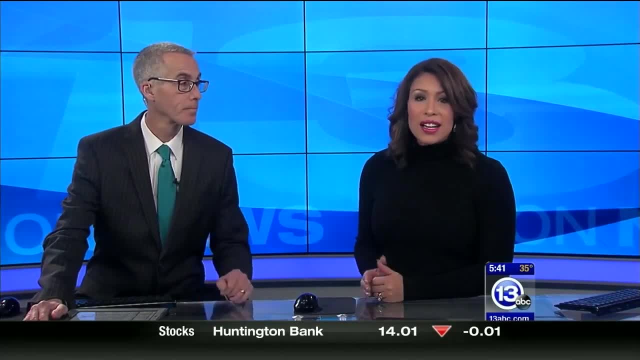 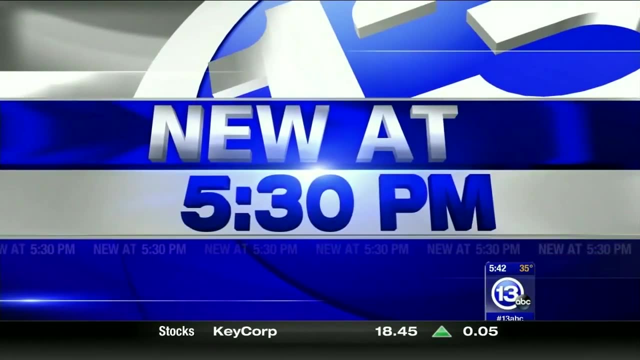 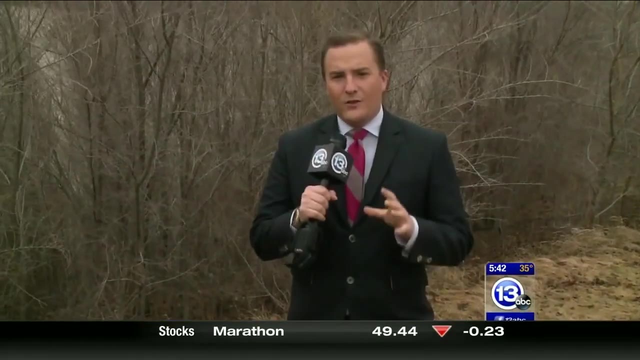 Well, federal climate experts seem to all agree. last year was the hottest on our record books across the globe. The third year in a row that record was broken. 13. ABC meteorologist Ben Cathy found that even if we don't see a melting glacier down the street, you'll still see big changes close to home. Those record highs. 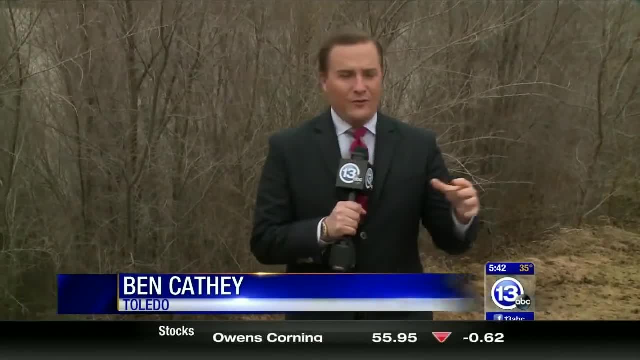 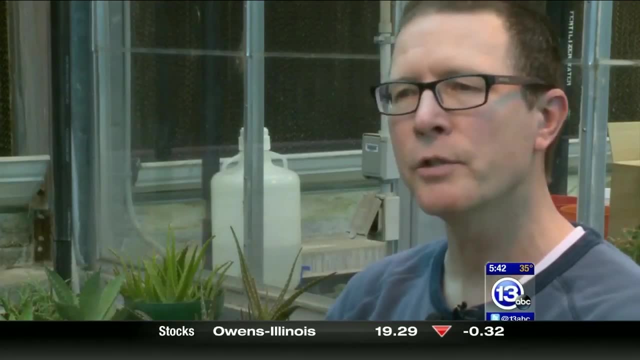 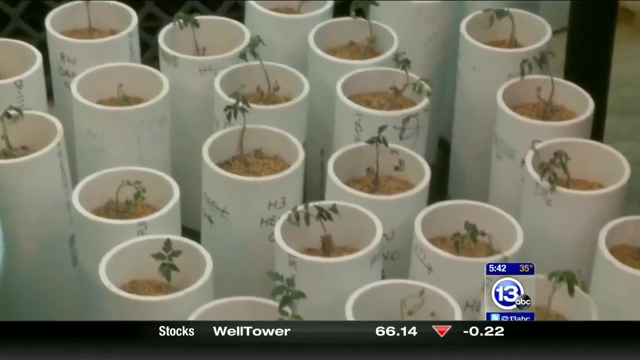 and increasing prolonged heat waves don't just mean less food from plants like tomatoes, but new research shows less nutritious food as well. That food will have a lower nutrient concentration. Dr Scott Hecathorn's team at UT studies crops like barley and tomatoes Now that summer standby may be in. 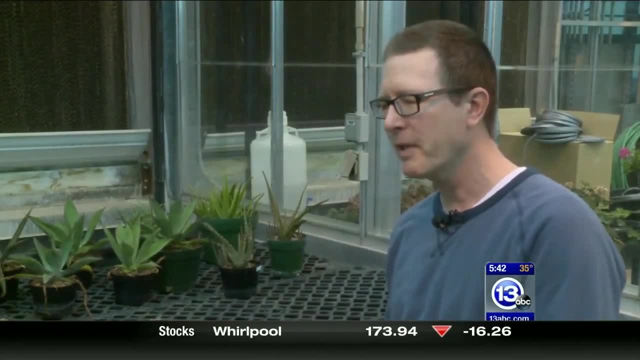 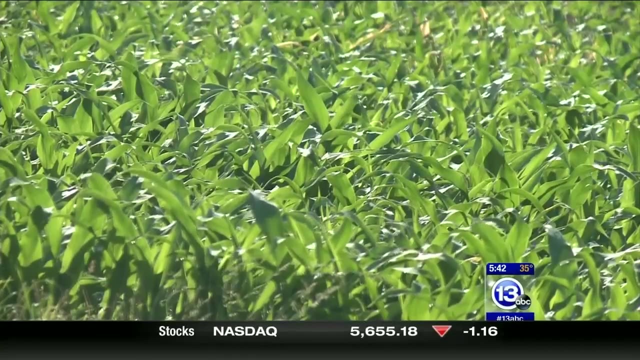 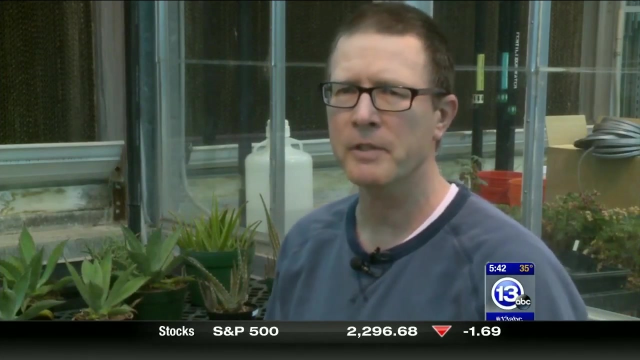 jeopardy Anybody who gardens with tomatoes. they know that tomatoes like it hot. They handle the heat, But it's a problem if it's too hot. Like people, plants can adjust to slow changes. However, what plants and other organisms have most to fear in a future world with global climate change is not the gradual. 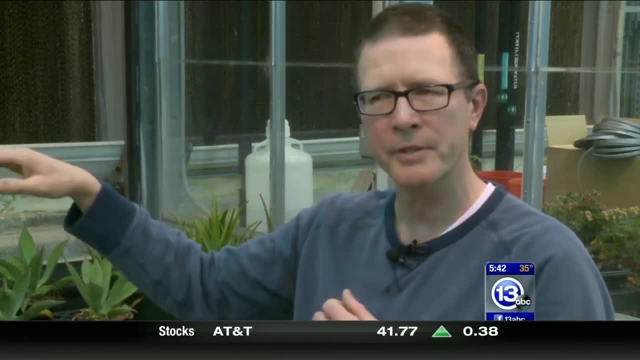 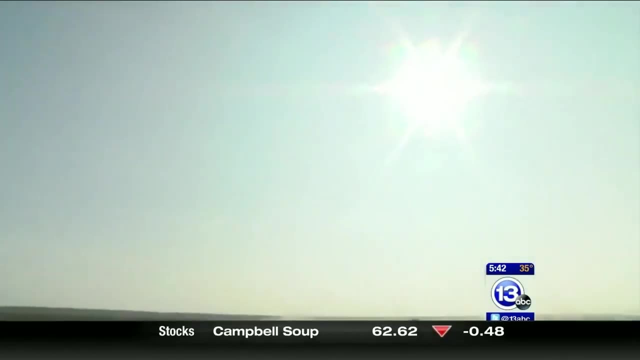 increases in temperature, but the increase in temperature. Or the gradual changes in precipitation, But those extreme events like droughts and floods and heat waves. While you may not know the impact of a changing climate every day, Professor Hecathorn says debate time is long over That evidence. 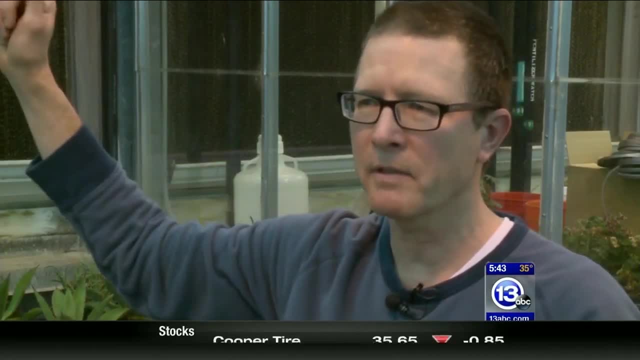 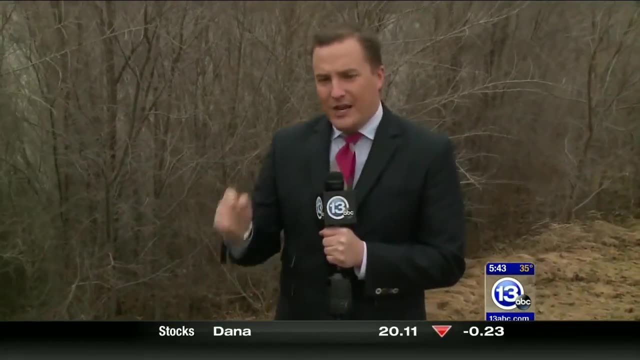 is indisputable. People who argue against that evidence are kidding themselves or they're not being honest. Local wildlife expert, Justin Grubb, has traveled all around the world seeing the effects of a changing climate on things like coral bleaching, And now he's seeing changes in his own backyard. The climate thing is something. 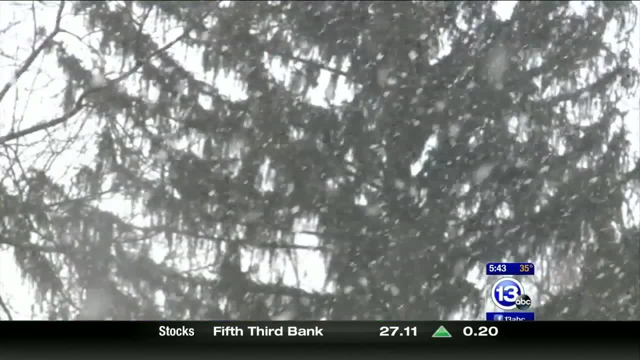 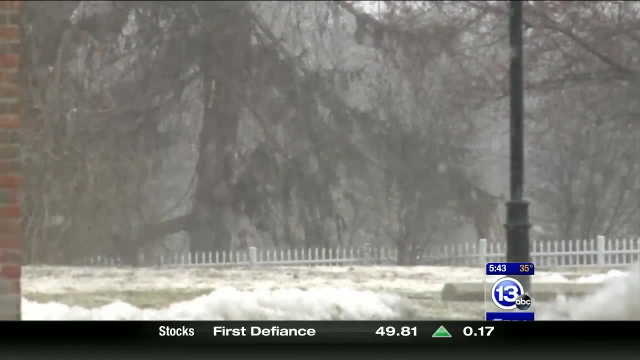 that we're observing almost immediately. Local animals woke up too early from hibernation during some recent winters. After a quick cold snap and with no food supply, some die off. I was going around in the field looking for amphibians and turtles and I was seeing a lot of dead animals kind of floating around in the